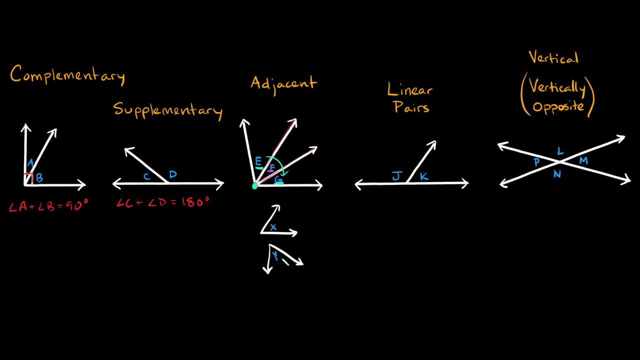 angle X and this is angle Y. okay, Are these adjacent angles? No, they're not right, Because I mean, I guess they're technically next to each other but, as you can see, they have completely different vertexes, right? So these are just two completely different angles, right? So that's one. 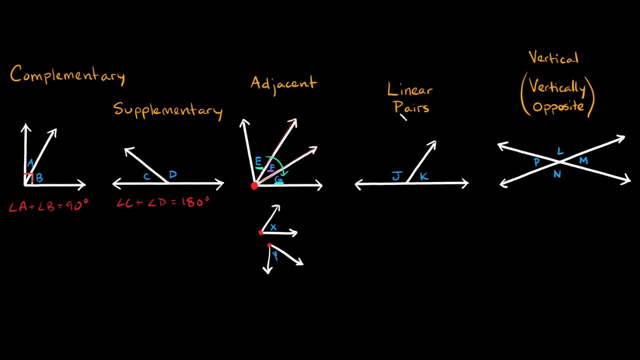 key point: they have to have the same vertex. right there Now linear pairs. So linear pairs are just adjacent angles, right? They're angles that are next to each other, that are supplementary, or in other words, they add up to 180 degrees. okay, So they're not next to each other, right? So they're. 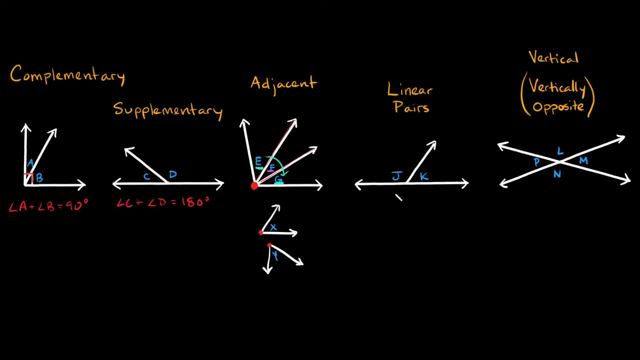 linear pairs, right, So these two angles right here, angle J and angle K, are linear pairs because, as you can see, they're next to each other, right, And they add up to 180 degrees. okay, So again, if I had something like this right here, right there, okay, that's good enough. So say: this is J and this: 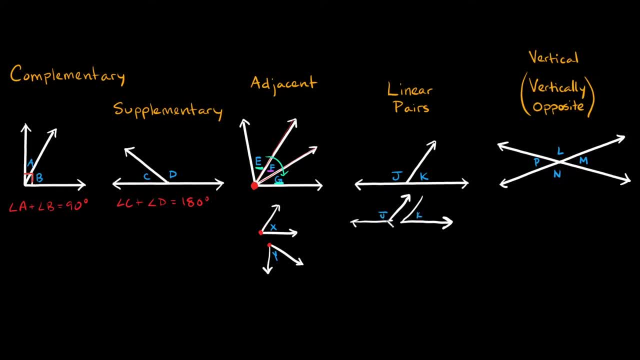 is K. Are these linear pairs right here? No, they're not okay, Because even if they do add up to 180, because again they have different vertexes here. Okay, now let's talk about vertical angles. So again, sometimes they're called vertically opposite angles, but really the easiest way to remember. 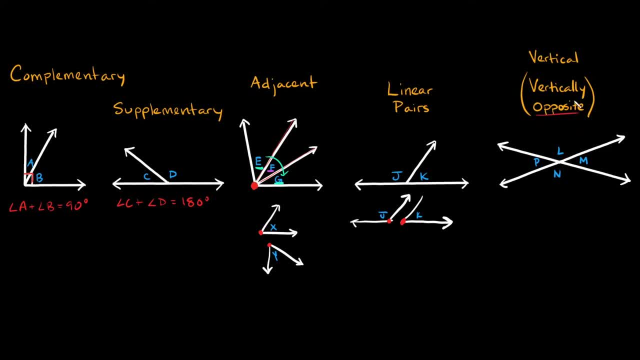 them is just by calling them opposite angles. okay, They're created by the same two intersecting lines, So opposite angles in this case would be, so L and N would be opposite angles. The other thing that happens here is that these two angles are equal to each other, okay, Or in other words, they're 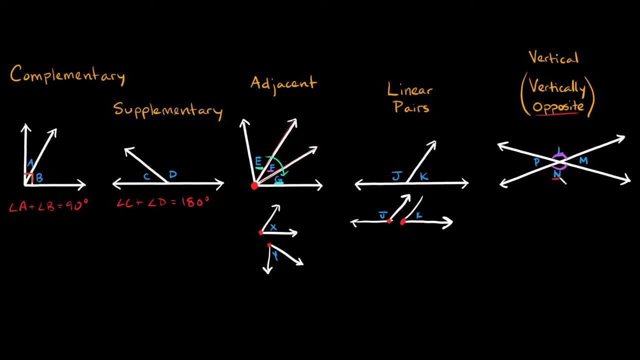 congruent to this angle. okay, They are the exact same angle. And then that happens with this other opposite pair over here, P and M. So this angle right here is congruent to this angle right here. okay, They're equal to each other, All right. so now that you have kind of an idea of what each of 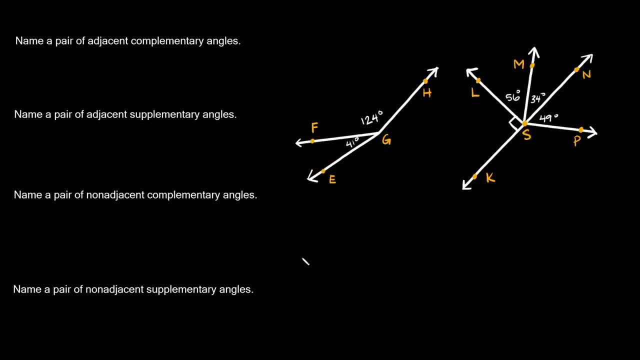 these are. let's just go over a couple examples to really tie it all together. All right, here's our first problem and these are the two figures that we're going to be referring to, all right, So first one says name: a pair of adjacent commas. 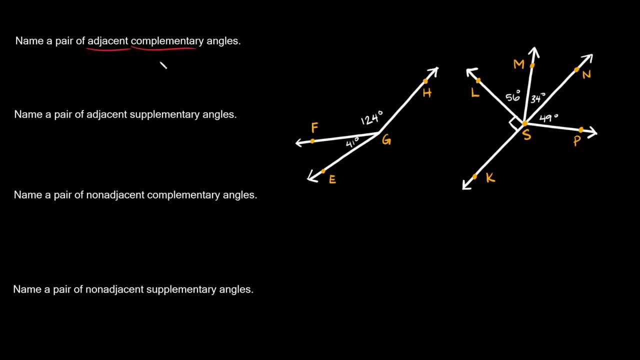 Complementary angles, all right. So remember, adjacent means next to Complementary, means they add up to 90 degrees, all right. So two angles that are next to each other that add up to 90 degrees, all right. So it looks like not these two, right, But it looks like this one, right here. 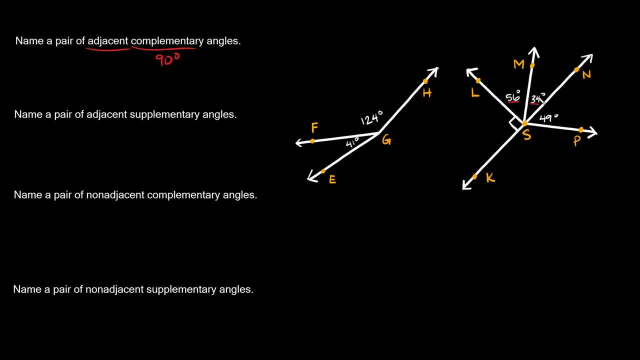 56 plus 34.. So 56 plus 34 is equal to 90,. okay, So we know that this right here is a right angle. also okay, Because these two angles, LSM and MSN, add up to 90 degrees. Okay, so a pair of adjacent, complementary angles again would be these two right here, right. 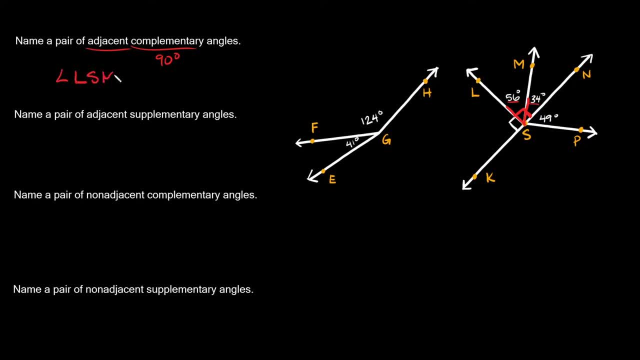 LSM. all right, Let's write that down. Angle LSM and angle. let's see the other one is angle MSN, right, Angle MSN, all right. So these are two adjacent complementary angles, all right. Now next one says: name a pair of adjacent supplementary angles, all right. So again, angles that are next. 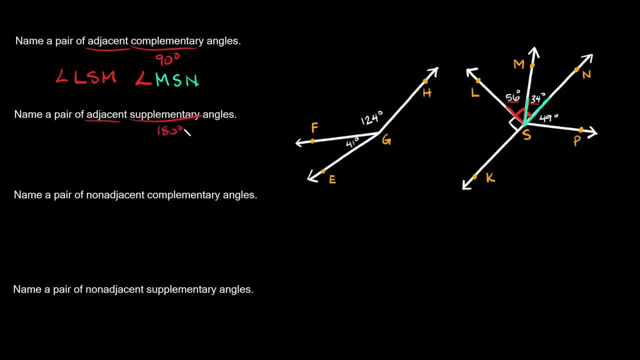 to each other and add up to 180.. degrees, all right. Well, let's see these two angles right here. looks like they add up to 165, so that's not it, okay? Well, if you notice, we have a straight line right here, right, KSN? So 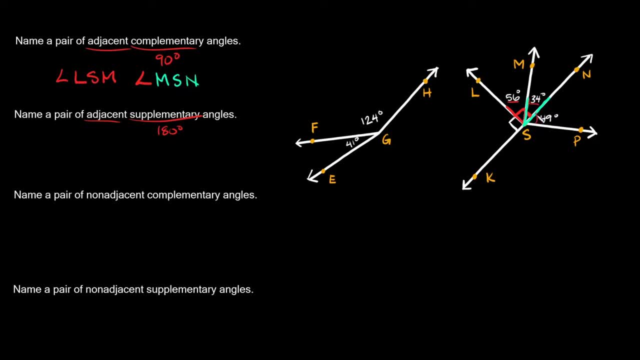 one thing that stands out is that this angle right here, this 49 and this angle right here are supplementary angles. okay, So again, that just means these two angles right here should add up to 180 degrees, right? So what should this angle be right here? Well, to figure that, 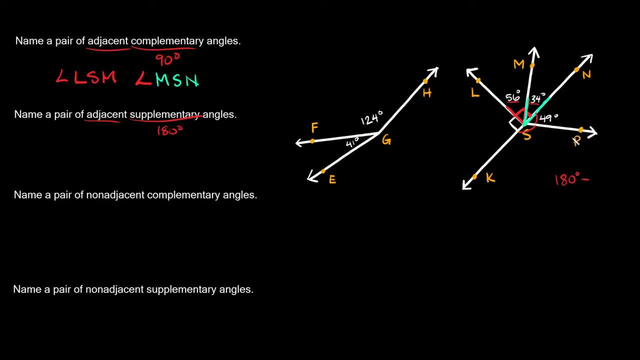 out. we would just have to do 180 degrees minus 49.. 49 degrees and that's equal to 131 degrees. right, So this angle right here is equal to 131 degrees. all right, So name a pair of adjacent supplementary angles. Well, in this case, we could do these two angles right here. right So NSP. 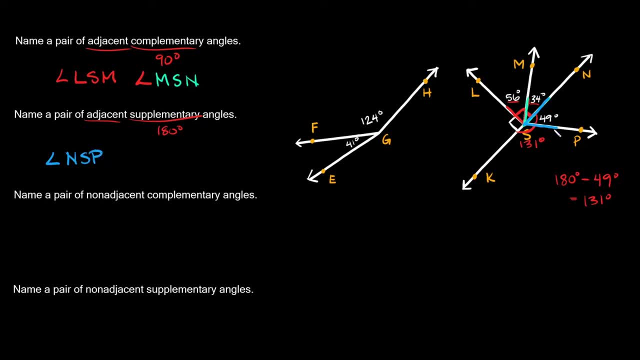 so angle NSP and this other angle, PSK. right So angle PSK. Those are adjacent supplementary angles. right Now, this one says: name a pair of non-adjacent complementary angles, okay, So in this case we're looking for angles. 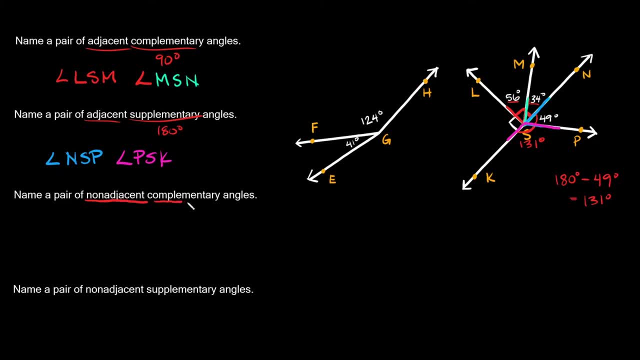 that are not next to each other, but they add up to 90 degrees, okay. So this one's a little tricky, but the two angles would be: this one right here, 41, and this angle over here, 49, right, Because 41 plus 49 is equal to 90, right. So two angles that are 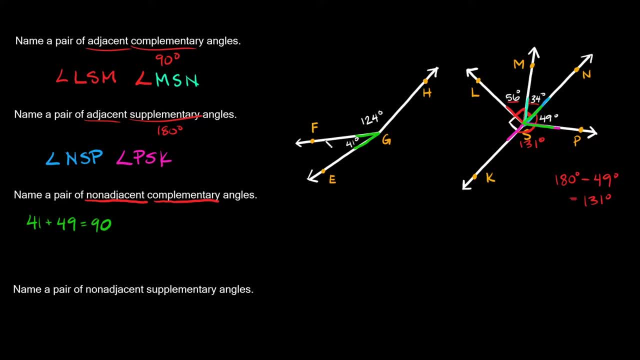 not next to each other, but they add up to 90 degrees would be FGE, right, So angle FGE. and this other angle over here, NSP, right, So angle NSP. okay. Now this last one says name a pair of. 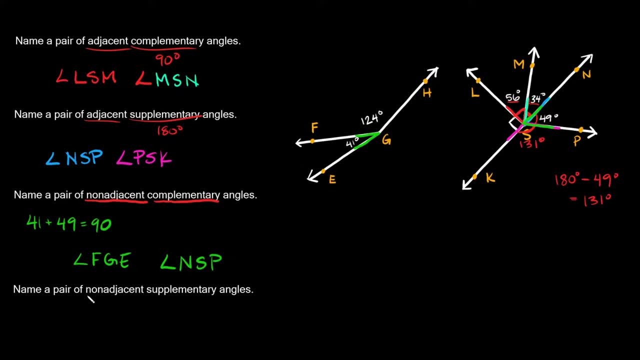 adjacent supplementary angles, right? So in this case, again, we're looking for angles that are not next to each other and they also have to add up to 180 degrees. okay, So here it would be these two angles right here. okay, This 124 and also this 56 right here? okay, Those two angles, right. So 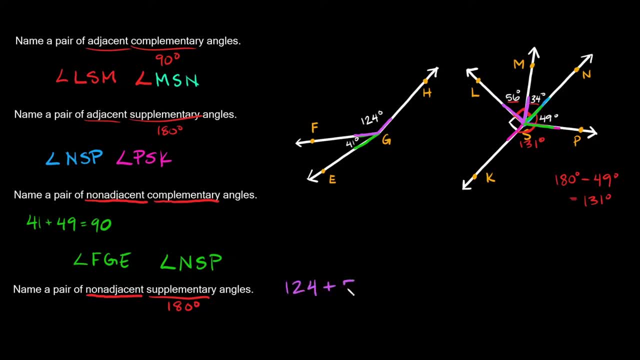 we'll just write it right here: 124 plus 56 is equal to 124, right, So these two angles would be 180 degrees, okay, So it'd be angle FGH, right Angle FGH and angle LSM, right LSM. all right, So. 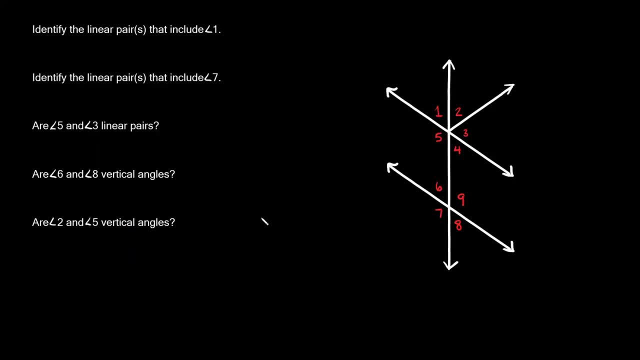 hopefully those weren't too bad. Let's try one last example. All right, so here's the last example, and this is the figure that we're going to be referring to. all right, So this one says: identify the linear pairs, or pair that includes angle one. okay, So angle one is right here. all right, So 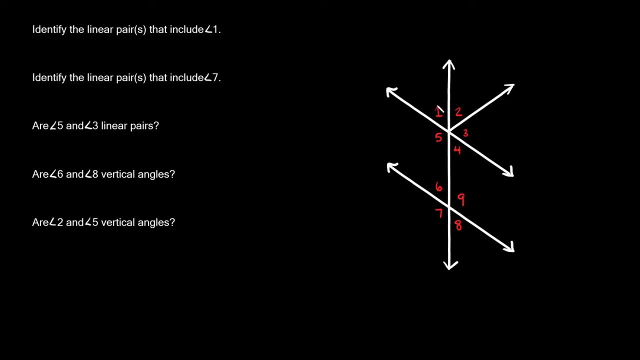 remember, linear pairs are two angles that are next to each other and are supplementary. all right, Or in other words, they add up to 180 degrees, right? So those always occur where there's straight lines. okay, So here, right, Here's angle one, So we can see one and five would be a linear pair. 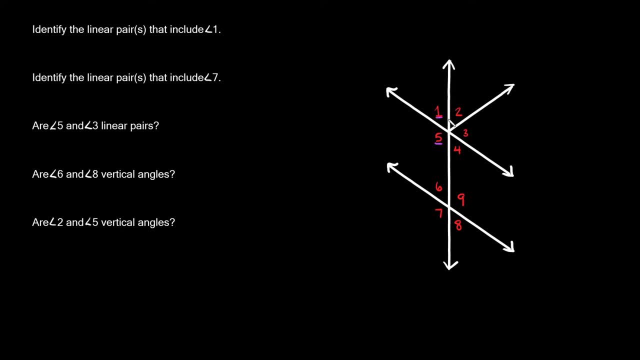 right, Because these two angles are next to each other and they are supplementary, right, These? this whole thing adds up to 180 degrees, okay, So here we could say that angle one and angle five are linear pairs or a linear pair. okay, Do we have any other linear pairs here? Could you say? 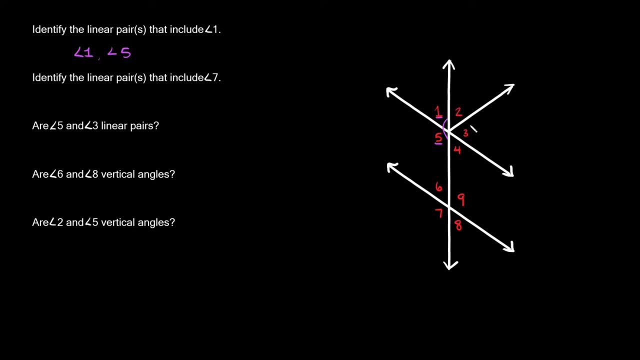 that one is a linear pair with angle two and three. No, because we're talking about pairs. right, Pairs come in two. This would basically be a triplet. So one, two and three, those are three different angles. right, That's not a pair, Even though these three right here do add up to. 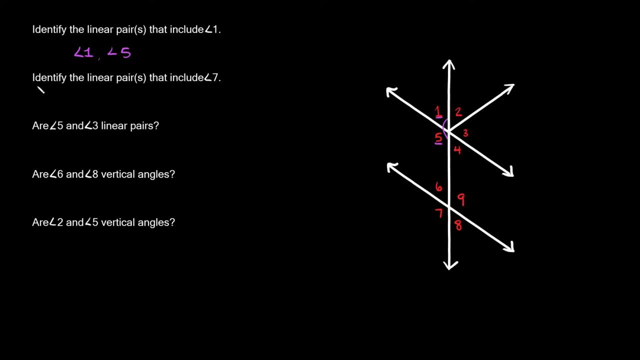 180 degrees. again, they're not a pair. okay, So let's go to the next one. So it says: identify the linear pairs or pair. that includes angle seven. all right, So here we have a linear pair, here's angle seven. okay, So in this case the linear pairs would be seven and eight, right? 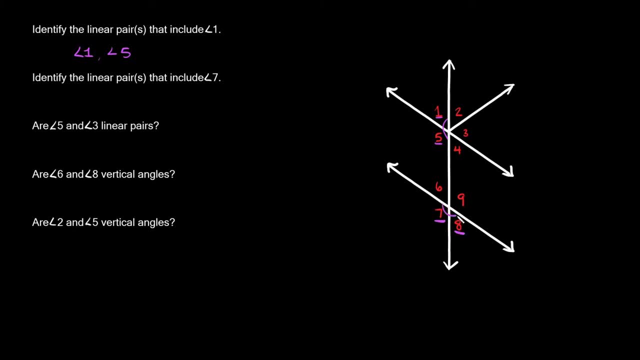 They're next to each other and they form this straight angle right 180 degrees. and seven and six are also linear pairs, right, Because these are next to each other and they also form this straight angle. right. These are supplementary angles, okay, So angle six and angle seven. 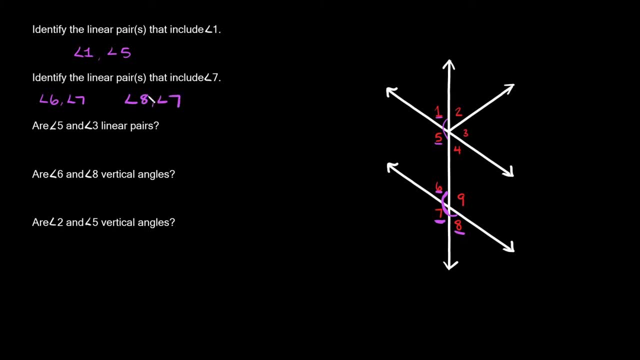 and angle eight and angle seven are also a linear pair. all right. Next one, So it says, are angle five and angle three linear pairs. Okay, so here's angle five, here's angle three. Are these next to each other? No, they don't even form, they're not even supplementary angles, right? They're not along. 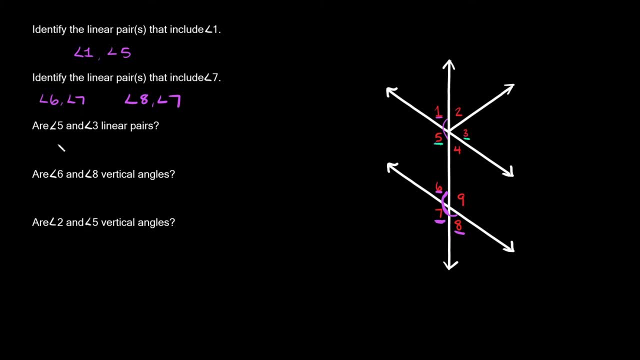 a straight line or anything like that. So these are definitely not linear pairs. okay. Now this one says: are angle six and angle eight vertical? Okay, so these are definitely not linear pairs. vertical angles- okay, Remember vertical angles. another way to think about them is by calling: 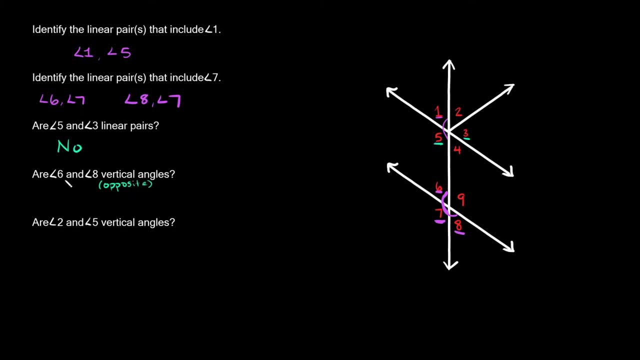 them opposite angles, opposite, Okay. so six and eight. So here we have six, here we have eight, and they're formed by the same two straight lines, right here, right? So are these opposite angles? Yes, they are, which again means they're congruent angles. Okay, next one Are angle two and angle 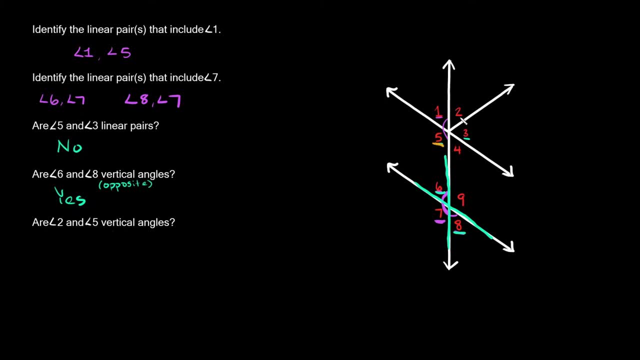 five vertical angles, All right. so let's see Angle five, angle two: Okay, are these vertical angles? Are they opposite angles? No, they're not okay. So a couple things you can see are: angle five: this is a big obtuse angle right. Angle two: 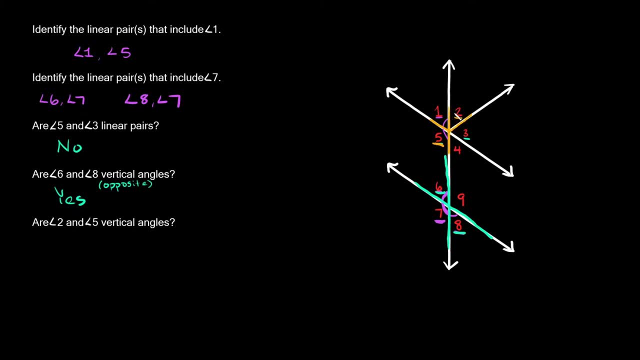 over here is an acute angle. it's a smaller angle, okay, So again, these are not the same angle. they are not congruent. The other thing is they're not formed by the same two intersecting lines. right, These two intersect to make number five, But, as you can see, number two over here.